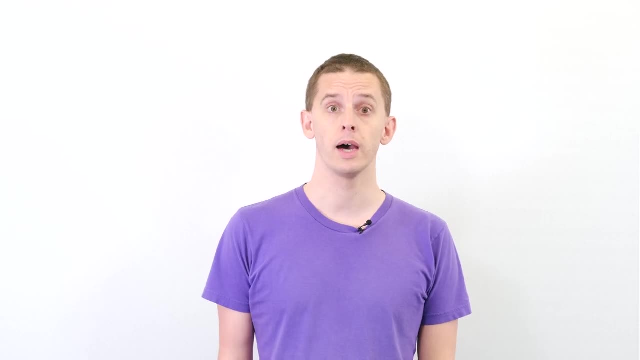 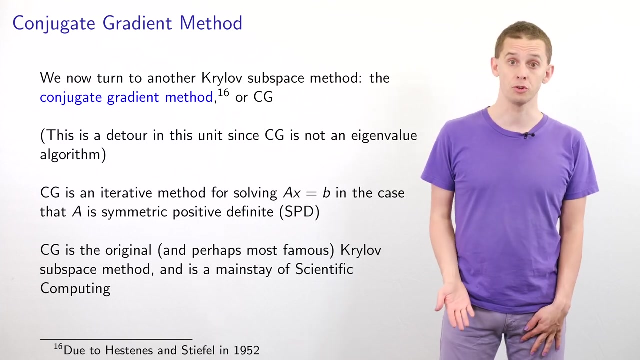 The conjugate gradient method has some interesting mathematical structure and is a very efficient way to solve a broad class of sparse linear systems. We now turn to another Krylov subspace method, the conjugate gradient method or CG, that was introduced by Hestien and Steiffel in 1952.. 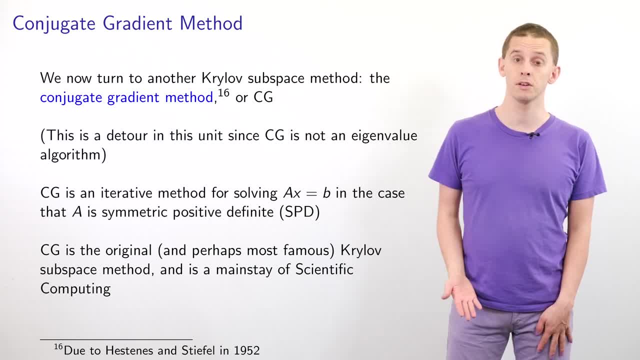 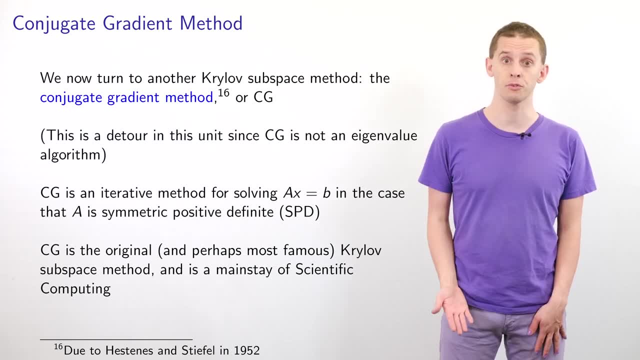 And CG is an iterative method for solving linear systems: ax equal b in the case when a is a symmetric positive definite matrix. that we often abbreviate as SPD. CG is the original and perhaps most famous Krylov subspace method, and it is a mainstay. 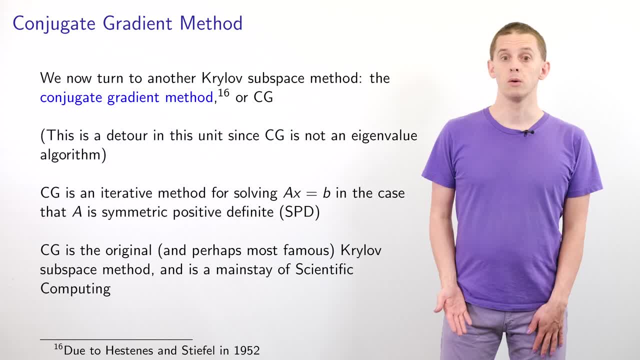 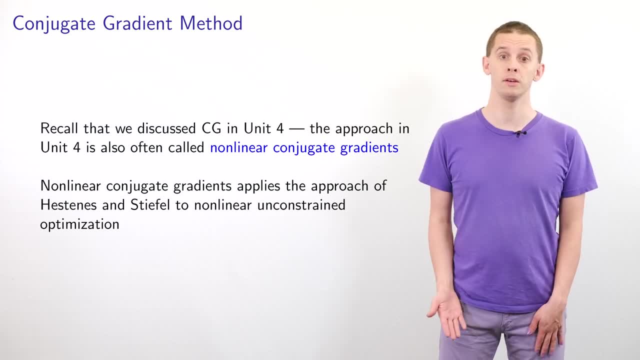 of scientific computing. We briefly discussed CG in Unit 4, and the approach in Unit 4 was called nonlinear conjugate gradients, And this is an algorithm that applies the approach of Hestien and Steiffel to nonlinear unconstrained optimization And at the time we just presented 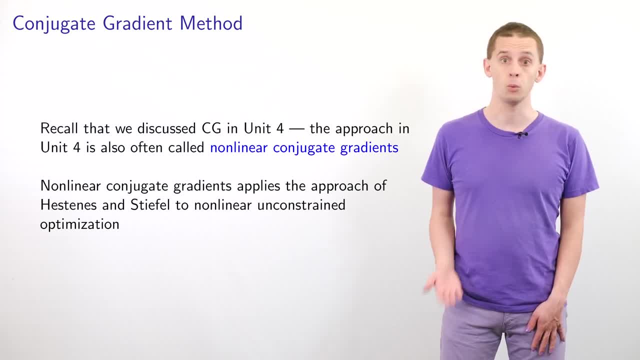 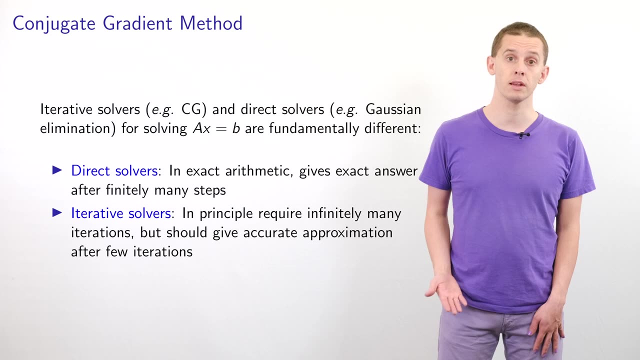 the algorithm and we did not talk about where it came from, And so here we're going to look in detail at how exactly these algorithms work. So iterative solvers like CG, and direct solvers like Gaussian elimination for solving linear systems ax equal, b are fundamentally different With direct 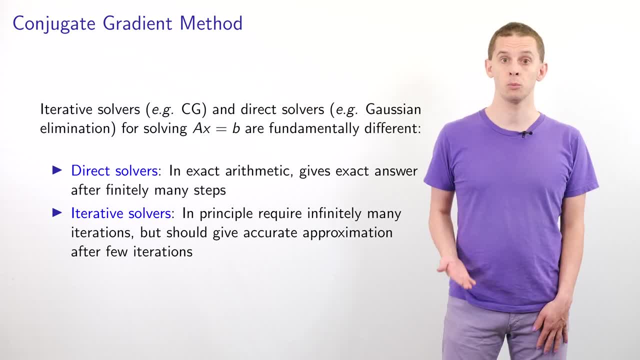 solvers. if we work in exact arithmetic, then we should get an iterative algorithm that is an exact answer after finitely many steps With iterative solvers. in principle they require infinitely many iterations, but they should give an accurate approximation after a few iterations. 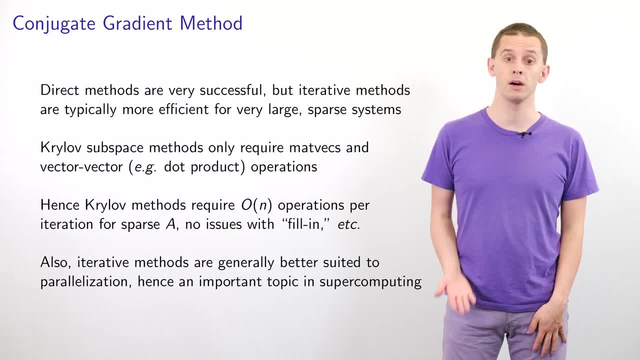 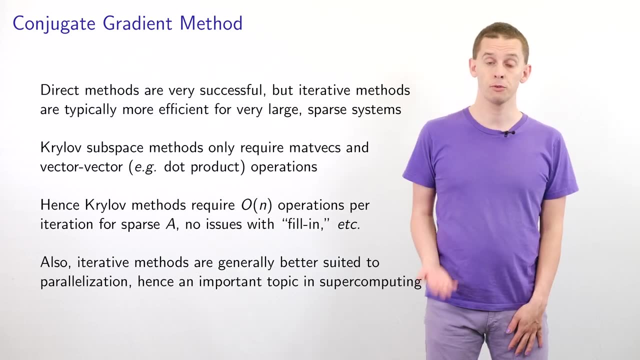 Direct methods are very successful, but iterative methods are typically more efficient for very large, sparse systems And Krylov methods typically only require matrix, vector multiplications or vector matrix And therefore if Krylov methods are working on a large, sparse n by n matrix, they would 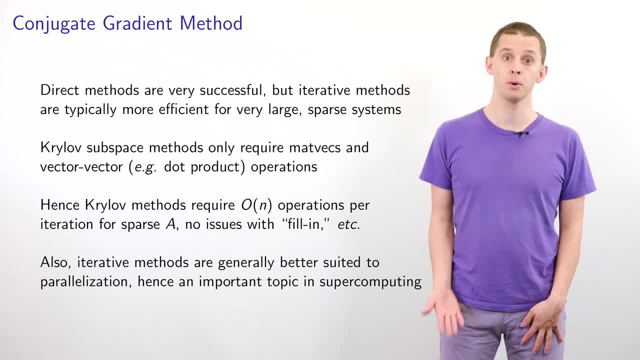 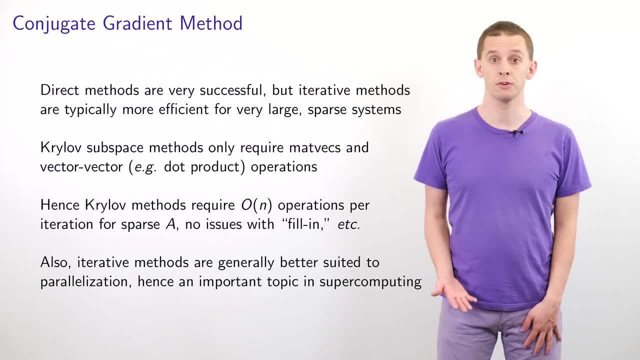 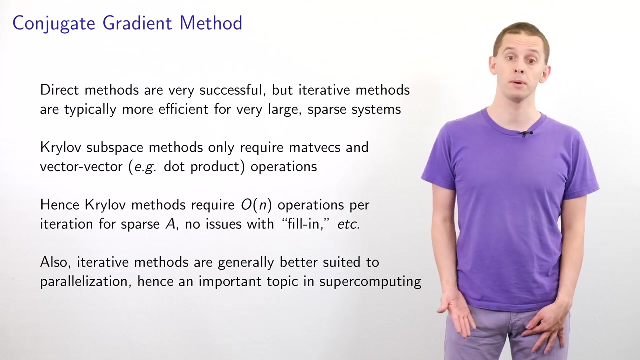 typically require big O of n operations per iteration And they don't suffer from some of the problems that direct methods have, For example fill in of sparse matrices that can happen in the LU factorization. In addition, iterative methods are generally better suited to parallelization and therefore they're an important topic in supercomputing. 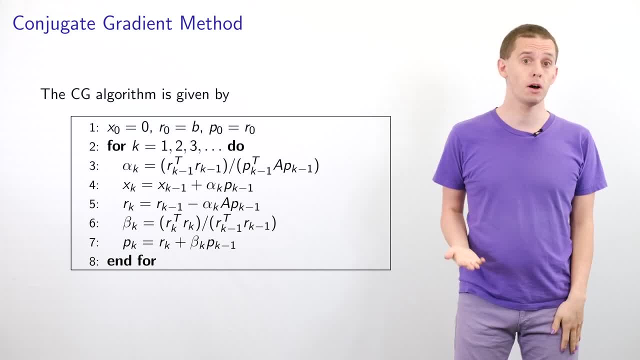 So let's now look at the CG algorithm. And it's certainly not obvious how this algorithm works up front, But we'll first get an overview of it before we look at how it works in detail. And the algorithm makes use of three sets of vectors. We have the vectors xk that are our 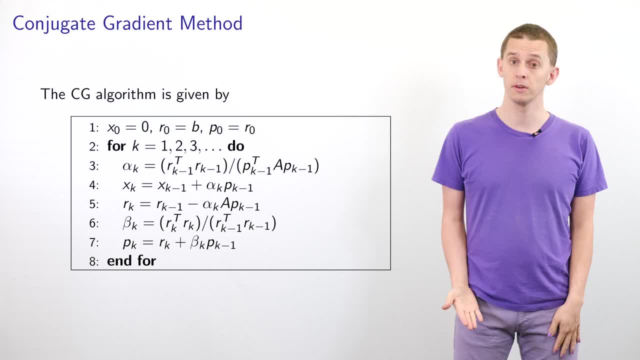 solution iterates, We have corresponding residuals, rk, And they're defined such that every stage rk is equal to b minus a of xk. And then we have directions that we update our solutions by pk, And in the algorithm we first compute a scalar alpha k. We then use that to 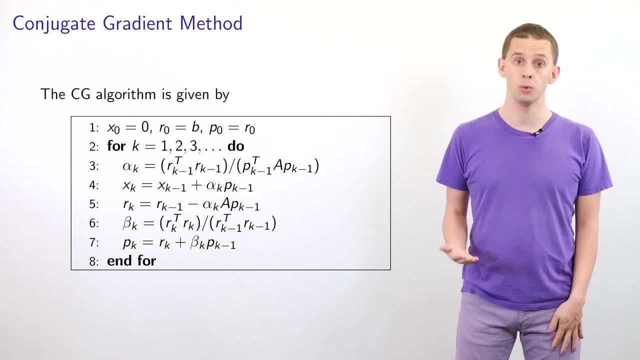 update our solution xk And we update the corresponding residual rk. We then compute a second scalar beta, k, And we use that to find the next direction, pk, that we will move in on the next iteration. So let's now look in detail at exactly how this. 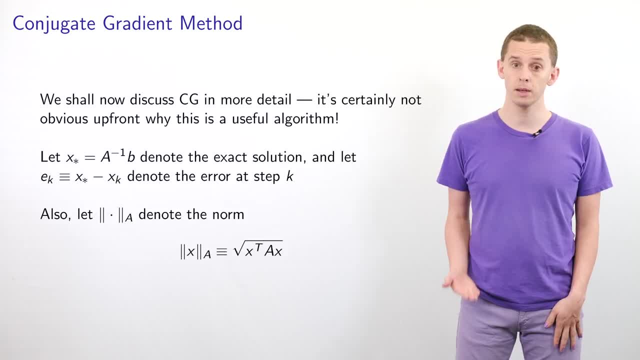 algorithm works And, to begin with, we're going to define x star equal to a inverse b as the exact solution to our linear system, and we can therefore write down that ek is the error at each step, which is equal to x star minus xk. We'll also introduce an a norm defined for a vector x to be the square root of. 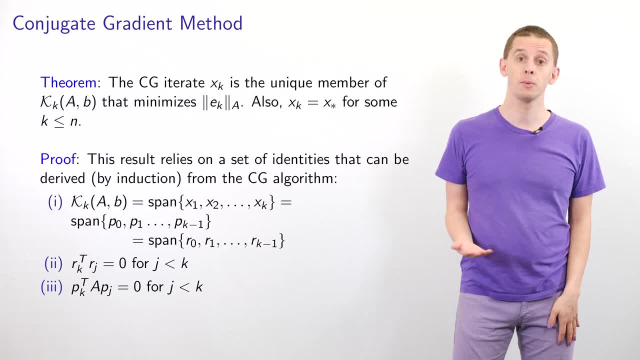 x transpose ax. So we now have a theorem that says that the CG iterate xk is the unique member of the Krylov subspace kk of ab that minimizes ek with respect to the a norm. In addition, we have that xk is equal to x star, for some k less than or equal to n, and the proof of this result relies on a set. 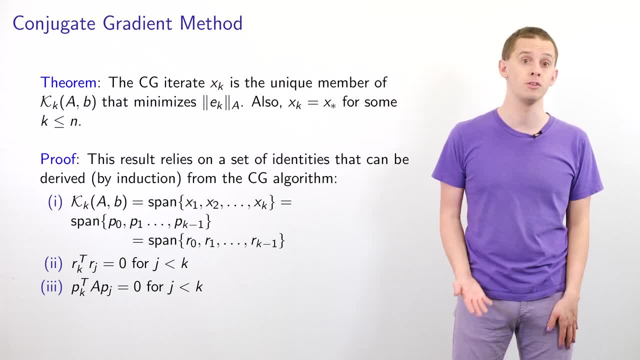 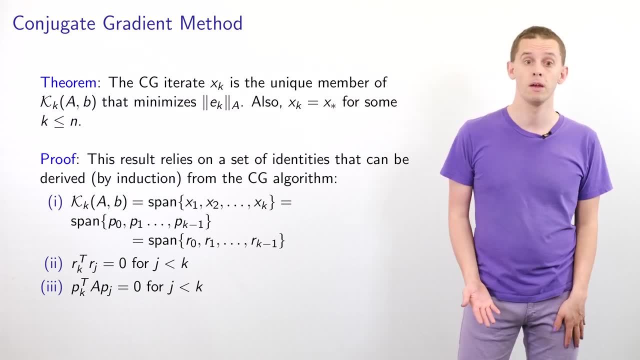 of identities that can be derived by induction from the CG algorithm. The first identity is that kk of ab is equal to the span of the vectors x1 to xk. and the first identity is that kk of ab is equal to the span of the vectors x1 to xk. 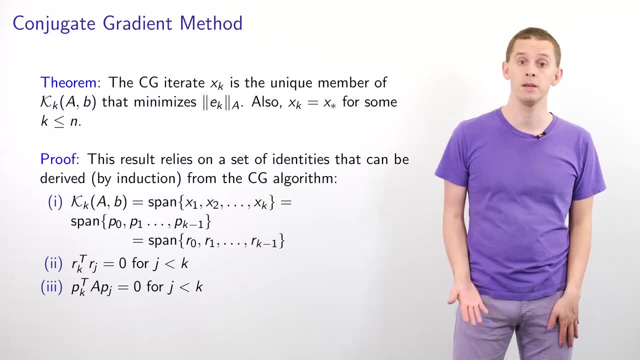 and the first identity is that kk of ab is equal to the span of the vectors x1 to xk. that's also equal to the span of the vectors p0 to pk minus 1 and is also equal to the span of the vectors r0 to rk minus 1.. The second identity is that rk transpose rj is equal to 0 for j less than. 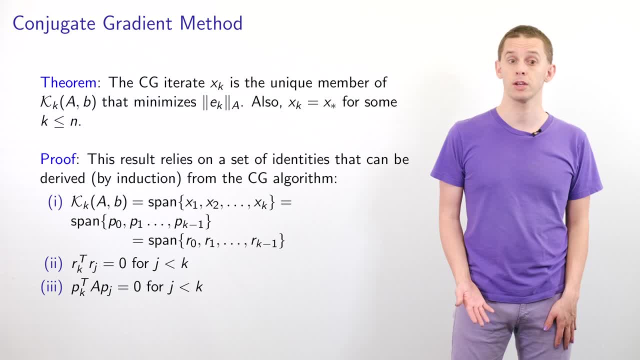 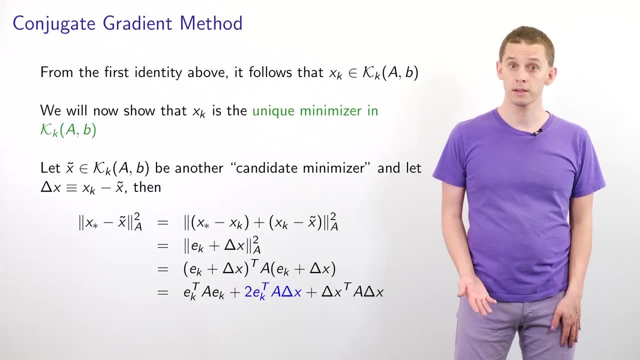 k and the last identity is that pk transpose apj is equal to 0 for j less than k. From the first identity above it follows that xk is in the Krylov subspace kk of ab and will now show that xk is the 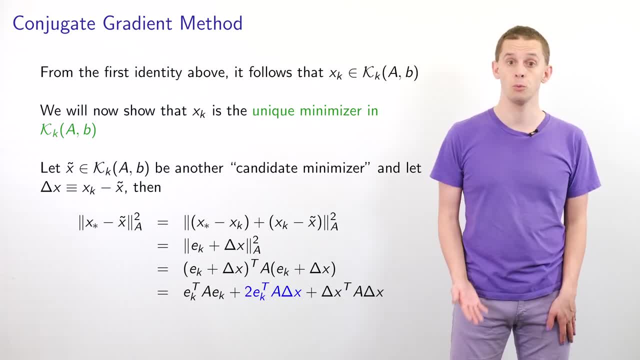 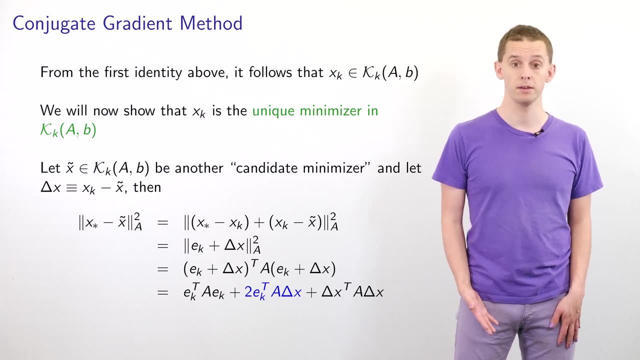 unique minimizer of ek with respect to the a norm in kk ab. To do this, let x tilde be another member of kk ab, that is, a possible candidate minimizer. and let's define delta x to be equal to x tilde, xk minus x tilde, the difference between the two points. So if we look now at the a norm squared of: 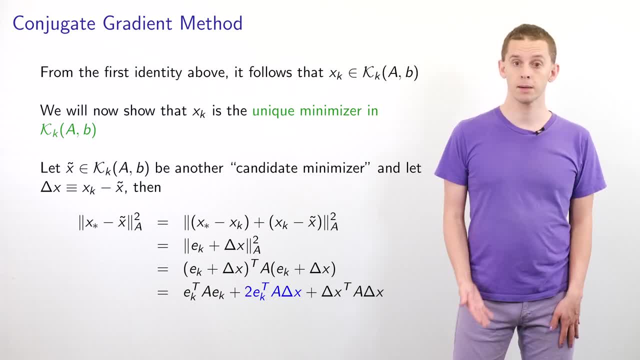 x star minus x tilde, then that can be written as the a norm squared of x star minus xk plus xk minus x tilde, and that can be written as the a norm squared of ek plus delta x, And by definition we can write this as ek plus delta x. transpose a ek plus delta x and we can. 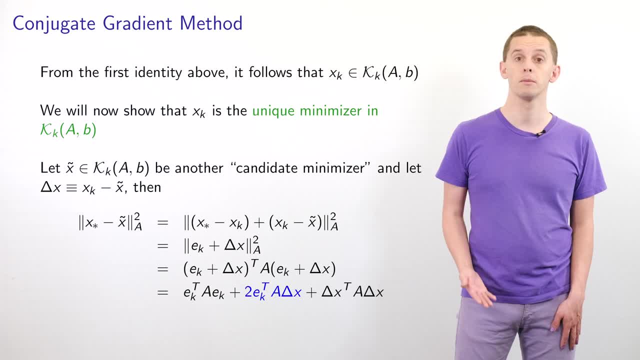 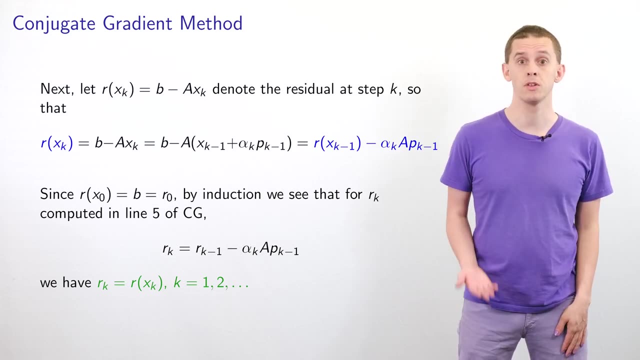 expand this out as: ek transpose a ek plus 2, ek transpose a delta x plus delta x transpose a delta x. Next, let r of xk be equal to b minus a of xk, which is the residual at step k. And we have that r of xk is equal to b minus a xk, which is equal to b minus a, xk minus 1 plus alpha k, pk minus 1. 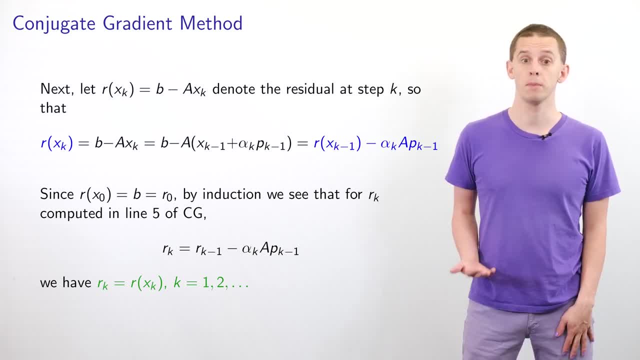 and that is equal to r of xk minus 1 minus alpha k, a pk minus 1.. We see in the initial setup of the algorithm that r of x0 is equal to b, which is equal to r0, and we also see by induction that. 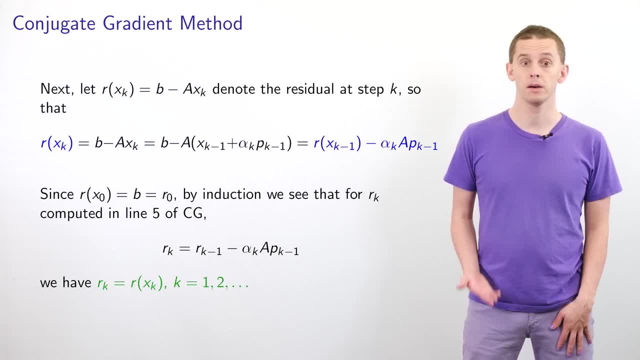 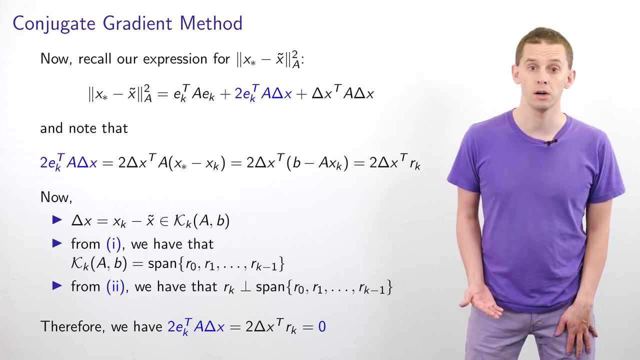 in line 5 of the cg algorithm, rk is equal to rk minus 1, minus alpha k, a pk minus 1, therefore confirming that rk is equal to r of xk for all, k equal 1, 2, 3 and so on. So now recall our expression for the: a norm: squared of x star minus x tilde. 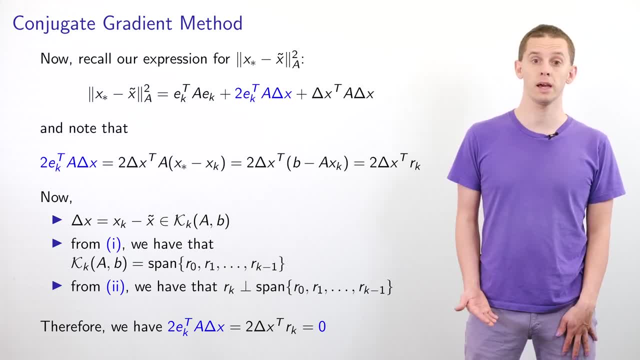 So that was equal to a norm squared of x star minus x tilde And this is equal to e k transpose a e k plus 2 e k. transpose a delta x plus delta x. transpose a delta x. And we can note that 2 e k transpose a delta x can be written as 2 delta x. transpose a x star minus xk. 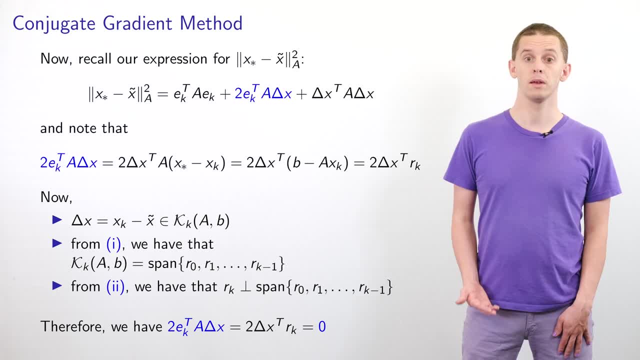 And that can be written as 2 delta x transpose b minus a xk, that is equal to 2 delta x transpose rk. So we know that delta x, which is equal to xk minus x tilde, is in the Krylov subspace, kkab, and from our identities we have that kkab is equal to the span. 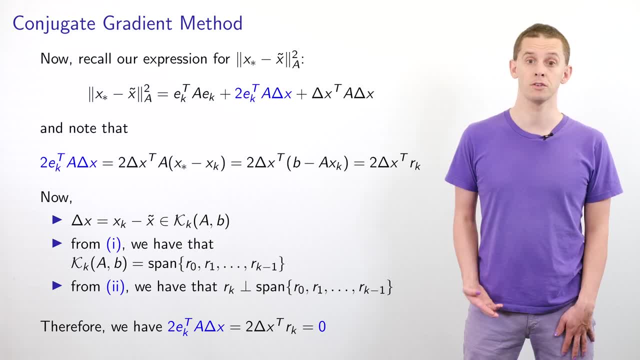 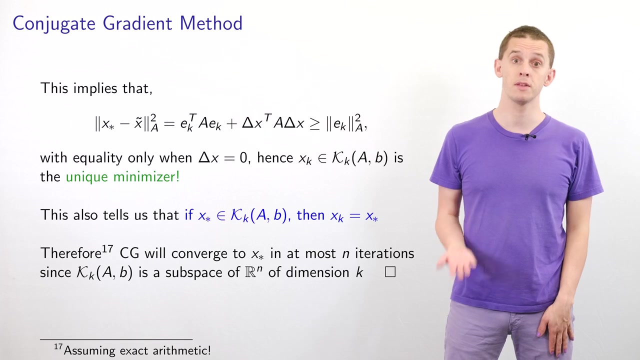 of the vectors r0 to rk minus 1, and we also know that from our identities that rk is perpendicular to the span of r0 to rk minus 1 and therefore we know that 2 ek transpose a delta x has to be equal to 0 because of that orthogonality relation. This implies that the anorm squared of x star minus x. 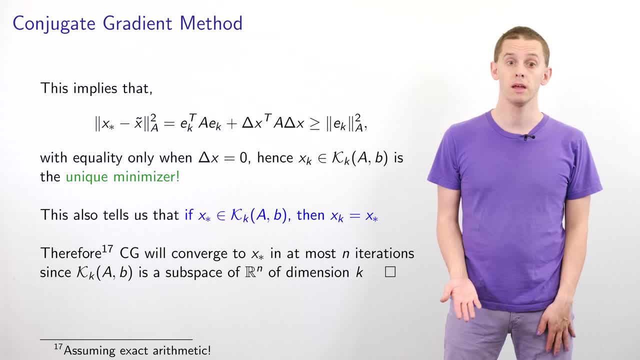 tilde is equal to ek. transpose a ek plus delta x. transpose a delta x and the first term here, that is just the anorm squared of ek. so we can therefore see this whole expression has to be greater than or equal to the anorm squared of ek, and we will only achieve equality in the case when 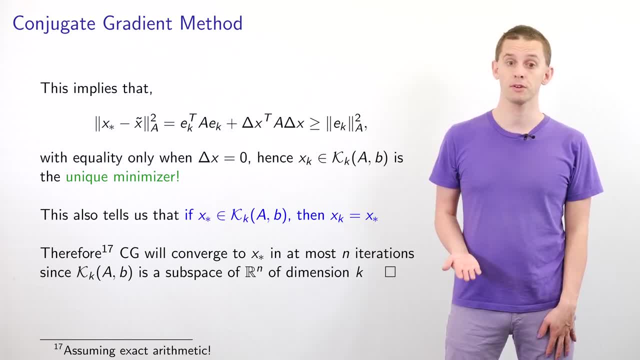 delta x is equal to 0.. So this therefore tells us, then, that xk is the unique minimizer within the Krylov subspace kkab that minimizes this quantity ek with respect to the anorm. This also tells us, then, that if x star is contained, 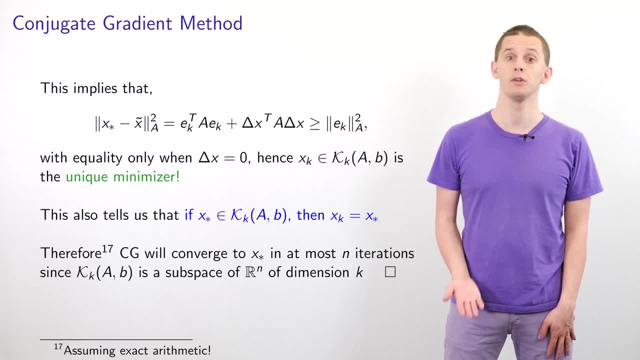 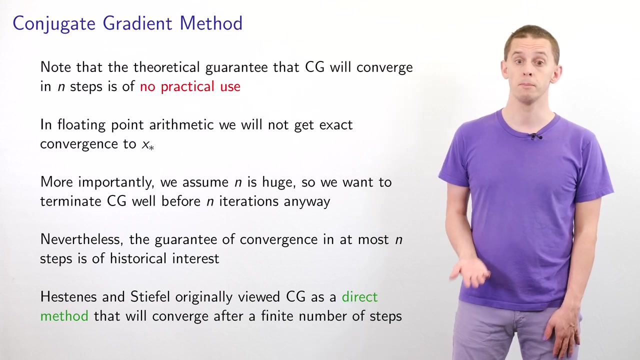 within kkab, then xk has to be equal to x star and therefore cg will converge to x star in most n iterations, since kkab is the subspace of rn, of dimension k. Note that the theoretical guarantee that cg will converge in n steps is of no practical use, because in floating point arithmetic we will: 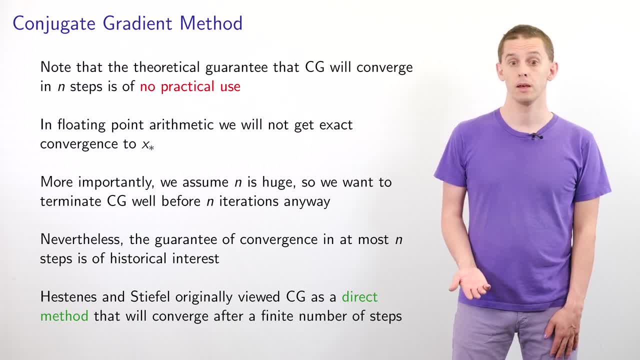 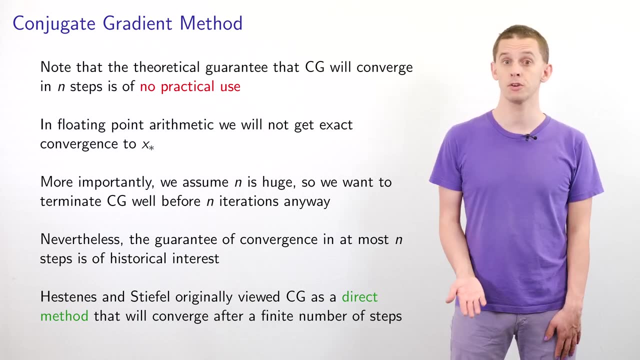 not get exact convergence to x star. More importantly, we assume that n is huge, so we want to terminate cg well before n iterations anyway. Nevertheless, the guarantee that you will have convergence in at most n steps is of historical interest and Hestien and Stiefel originally viewed cg as a direct method that 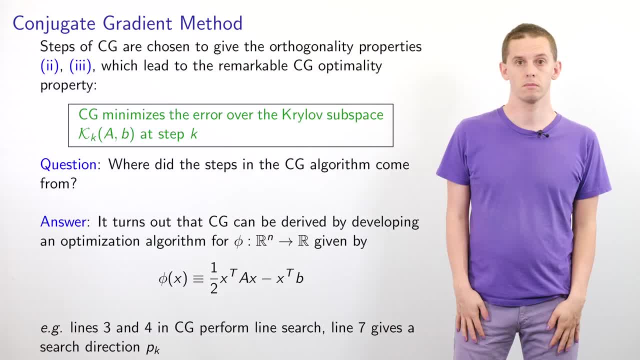 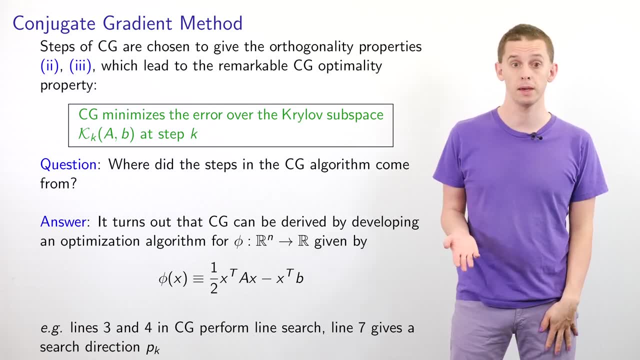 will converge after a finite number of steps. The steps of the cg algorithm are chosen to give the orthogonality properties for the rk and the kkab. So we can see that the convergence of n steps is the pk, which lead to the remarkable cg optimality property. that cg will minimize the error over the. 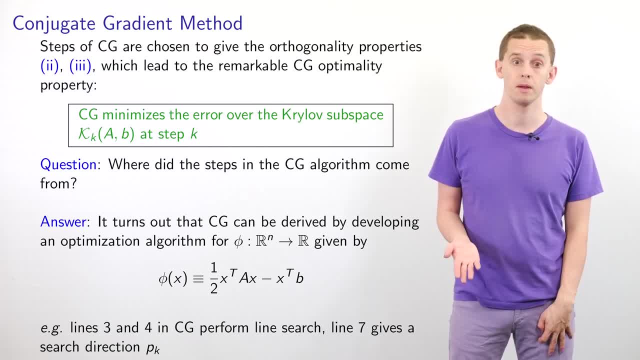 Krylov subspace, kkab at step k. So we might ask ourselves, where do the steps in the cg algorithm come from? And it turns out that cg can be derived by developing an optimization algorithm for the scalar function. phi from rn to r, given by phi of x, is equal to half x. 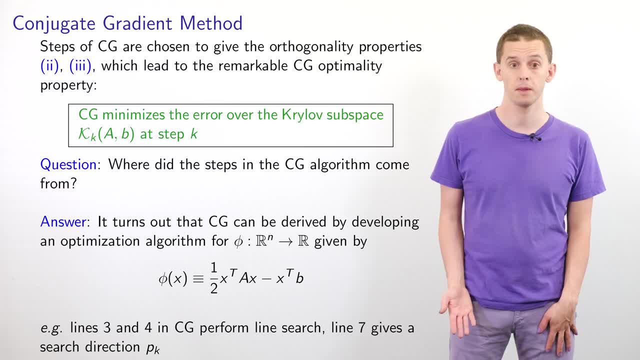 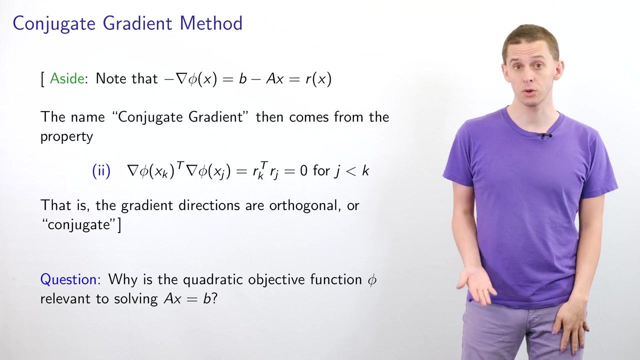 transpose ax, minus x, transpose b. And if we look at our cg algorithm then we find that lines 3 and 4 are performing a line search and line 7 is giving a new search direction. pk, As an aside, know that minus the gradient of phi is equal to b minus ax, which is just equal to r of x. 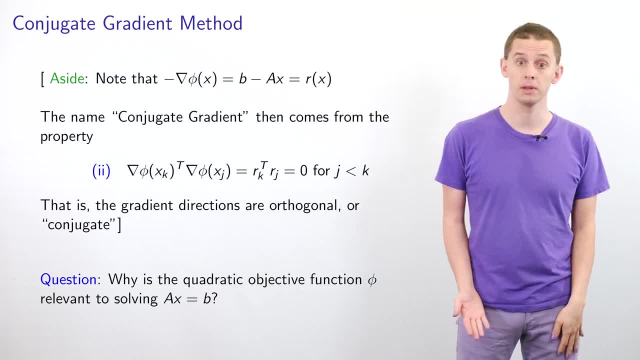 And the name conjugate gradient then comes from the property that if we take the dot product of gradients at two steps, xk and xj, that will just be equal to rk. transpose rj and that will be equal to zero for j less than k via our orthogonality relations. Therefore, the gradient directions are orthogonal. 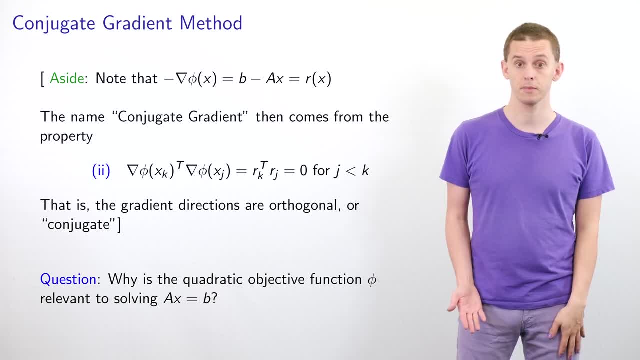 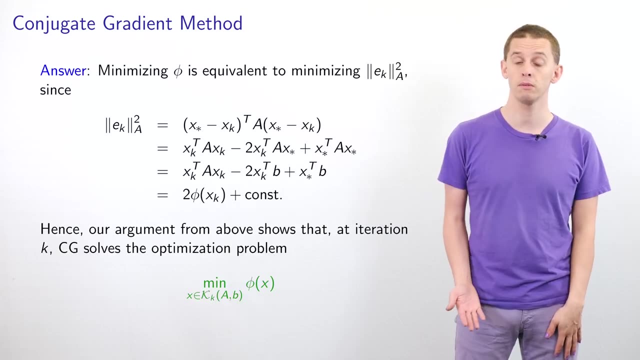 and we might also refer to them as conjugate. Now we can ask ourselves why the quadratic objective function, phi, is relevant to solving the linear system. ax equals b and the answer to this is that minimizing phi is equivalent to minimizing the anorm squared of Ek, Since if we look at the anorm squared of Ek, that will be: 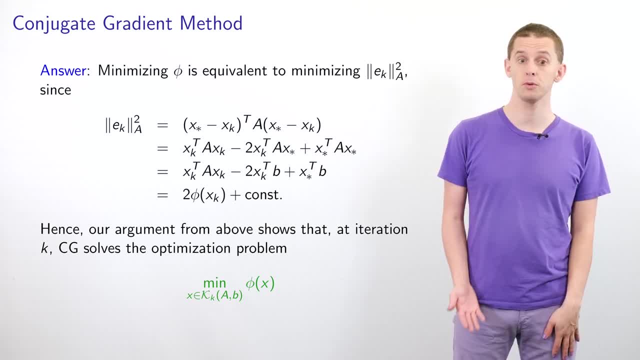 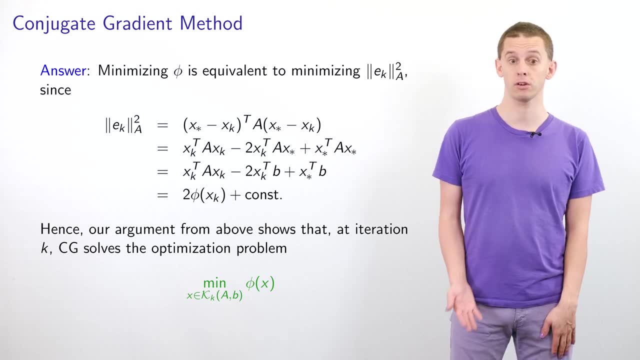 equal to x star minus xk. transpose a x star minus xk, which we can expand as xk. transpose times rk. A xk minus 2 xk. transpose A x star plus x star. transpose A- x- star, and that will be equal to xk. transpose A xk minus 2 xk. transpose B plus x star. transpose B and. 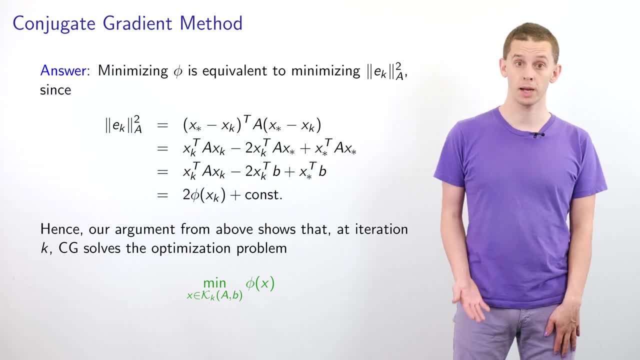 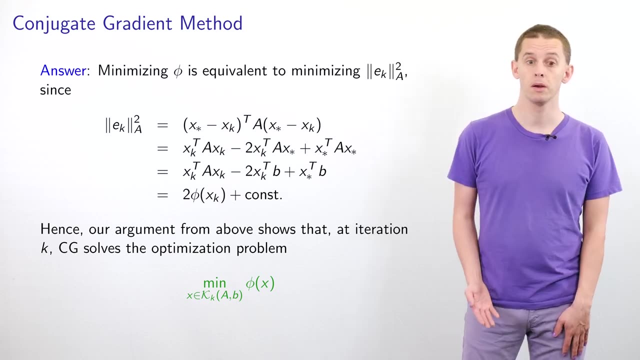 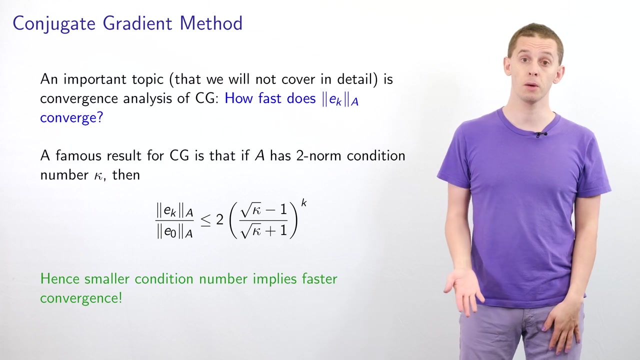 that will be equal to 2 times 5 xk plus a constant. Hence our argument from above shows that at iteration k, Cg is solving the optimization problem of finding the minimum over the Krylov subspace, kk of a, b, of phi, of x, An important topic which 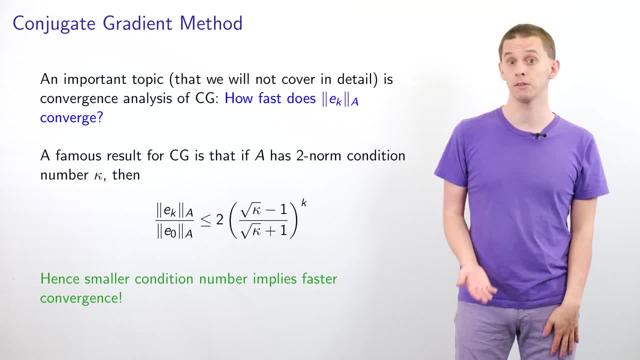 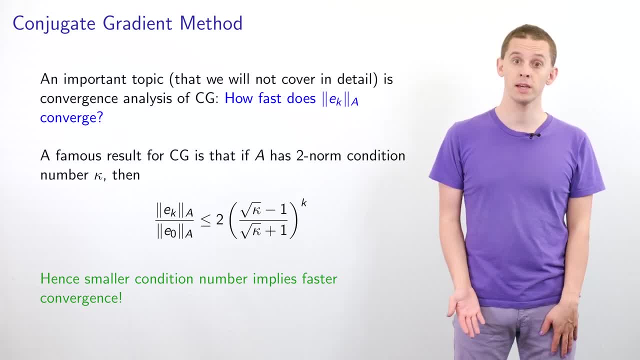 the power of kPa, then the A norm of ek divided by the A norm of E0 is less than or equal to 2 times the square root of kappa minus 1 divided by the square root of kappa plus 1 raised to the power of k, and therefore we see that smaller. 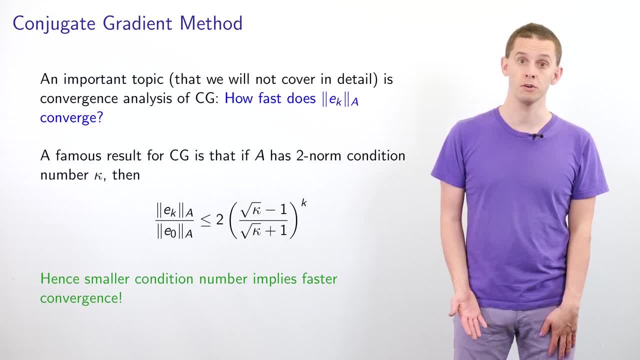 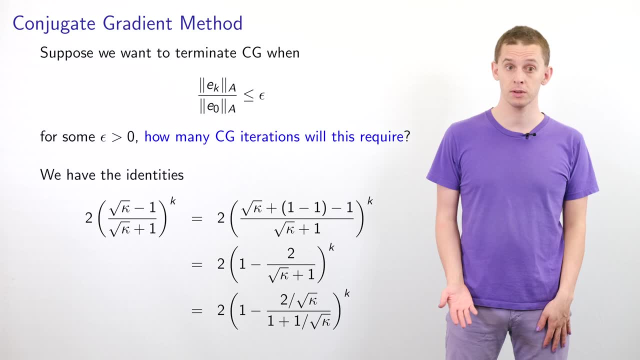 condition numbers will imply a faster convergence. Suppose we want to terminate Cg when the A norm of Ek divided by the A norm of E0 is less than or equal to e b micsilon, where epsilon is a small positive number. How many cg iterations will this require? 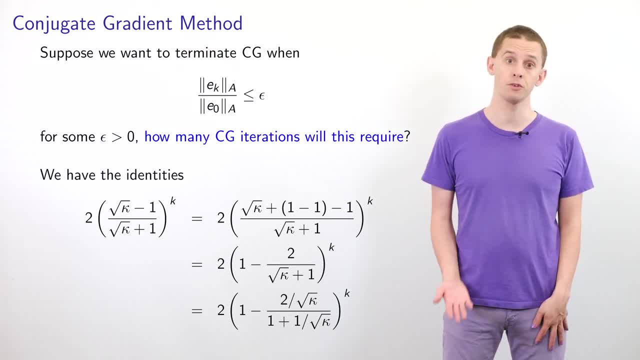 To answer this, let's look at the expression involving the condition number kappa. We have our expression: 2 square root kappa minus 1 divided by square root kappa plus 1, all raised to the kth power, and we can rearrange this to be equal to 2 times 1 minus 2 divided by the square root kappa. 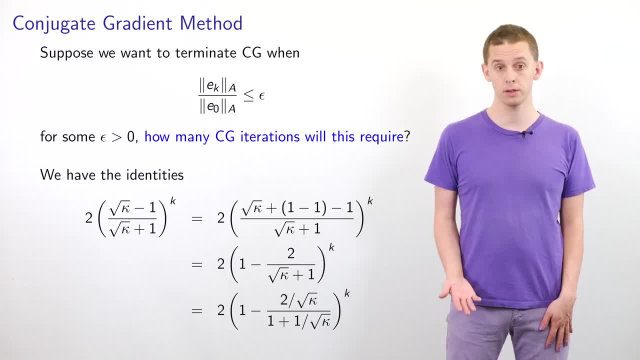 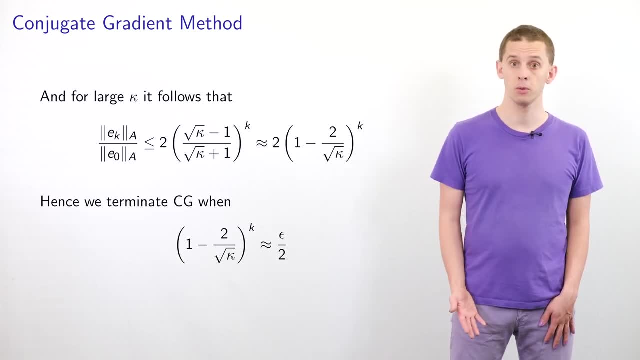 divided by 1 plus 1, divided by the square root of kappa, all raised to the kth power. and now let's look at the limit when kappa is large. In this case, the kappa factor in the denominator can be neglected and we therefore see that the anor vk divided by the anor v0 has to be. 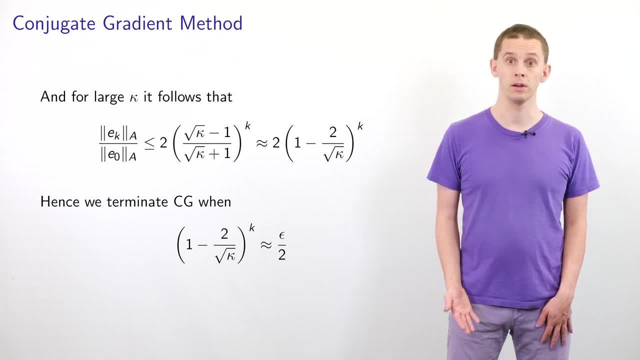 less than or equal to an expression approximate to 2k. Therefore we can terminate cg when 1 minus 2 over square root of kappa, all raised to the kth power, is approximately equal to epsilon over 2.. If we take logs of both sides then we see that k. 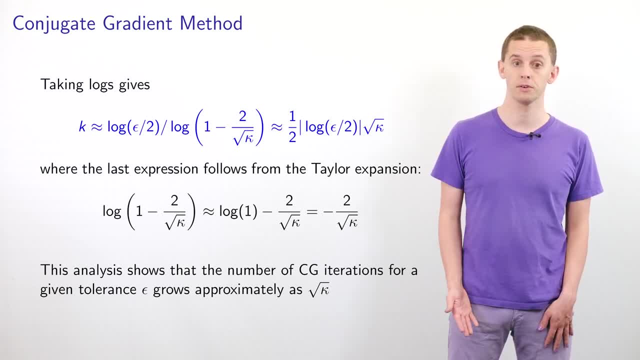 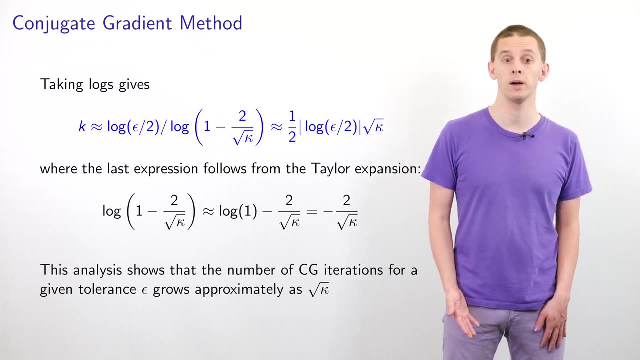 will be approximately equal to a half times the magnitude of epsilon over 2.. So this is the magnitude of the log of epsilon divided by 2 times the square root of kappa. And this last expression here follows from the Taylor expansion, where log of 1 minus 2. 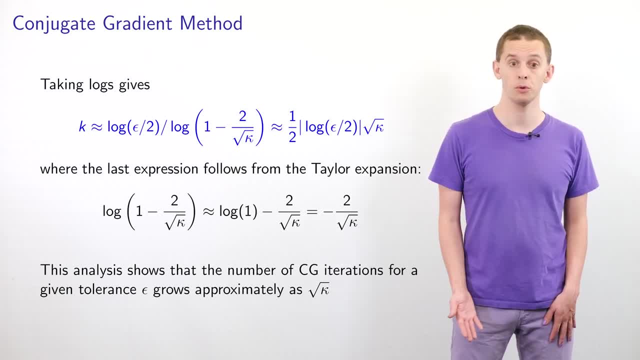 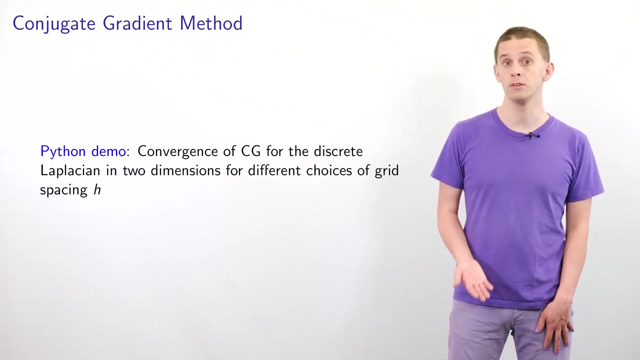 divided by the square root of kappa is approximately equal to minus 2 divided by the square root of kappa. So this analysis shows, then, that the number of cg iterations for a given tolerance epsilon will grow approximately as the square root of kappa. We'll now take a look at a Python example, where we use the conjugate gradient method to solve the discrete. 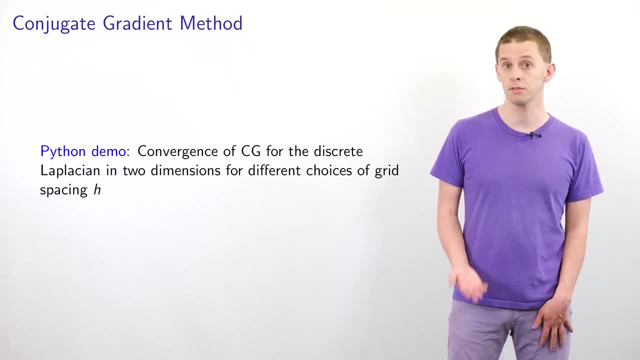 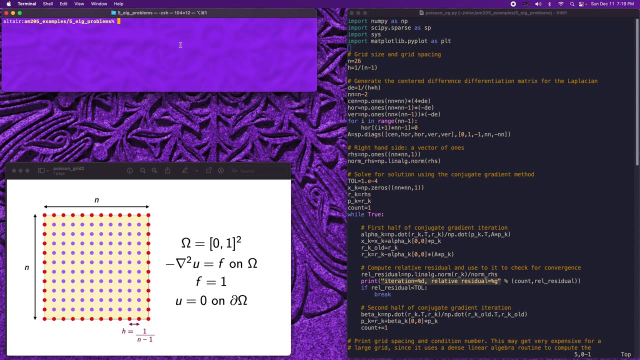 Laplacian on a 2D grid and we'll look at different sizes of grids and see how that affects the condition number and the number of cg iterations that we require. We'll now look at the program PoissonCgpy that demonstrates the conjugate gradient method applied to the Poisson equation. 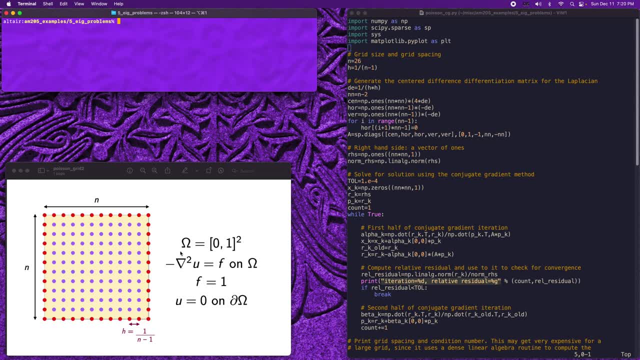 And we're going to solve the Poisson equation on the unit square, omega equal to 0,1 squared And the Poisson equation is: minus del squared, u is equal to f. on omega, And we're going to make use of a constant right hand side source term where f is just equal to 1 everywhere. 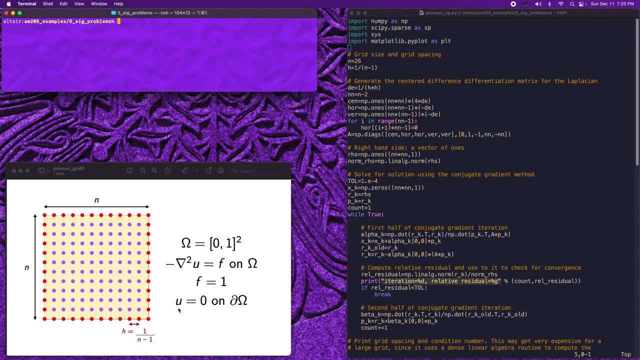 And we're going to use zero Dirichlet boundary conditions. so u is equal to zero on the boundary of omega And we're going to discretize omega using a regular square root of kappa And we're going to use a regular square n by n grid and that will correspond to a grid spacing of h equal to 1 divided by n minus 1.. 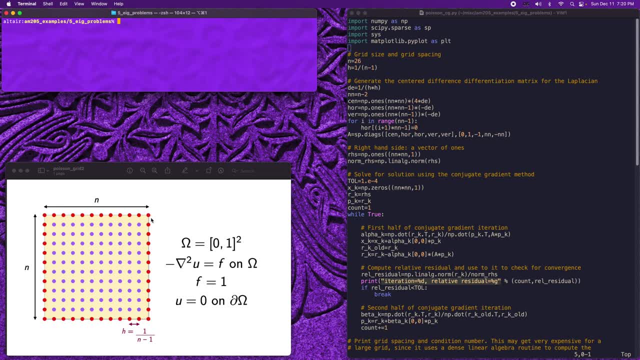 And in the diagram shown here the red grid points are on the boundary and our solution will be a zero there, And the purple grid points are in the interior and we need to solve for our solution there and it will be non-zero. If we look at the code, then we first define n. 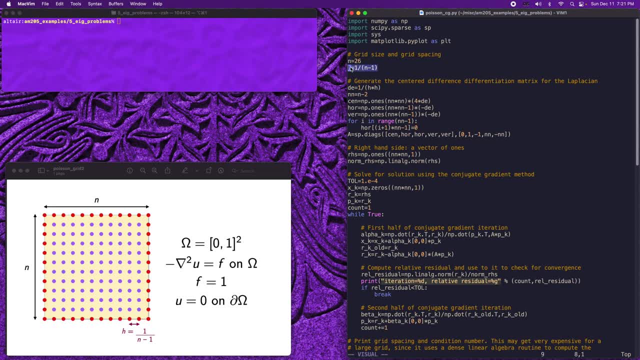 And here I'm going to use the Poisson equation- We're going to use a value of 26 and we then define the corresponding grid spacing. Next, we need to create the center difference differentiation matrix for the Laplacian, And we're going to make use of the standard five point stencil for the Laplacian. 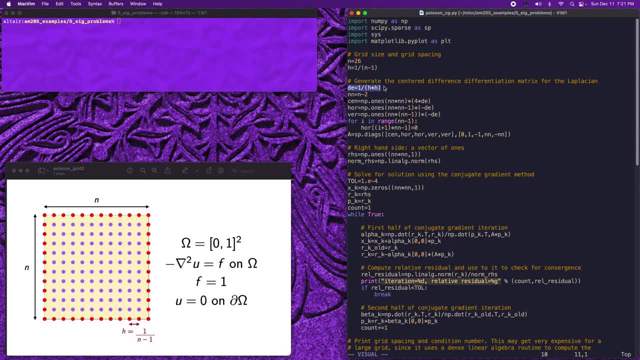 We'll define dE to be 1 divided by h squared, which is the term that appears in the denominator of the stencil entries, And we'll then define nn to be equal to n minus 2.. And that is the number of grid points across in the interior purple grid where we need to solve for our solution. 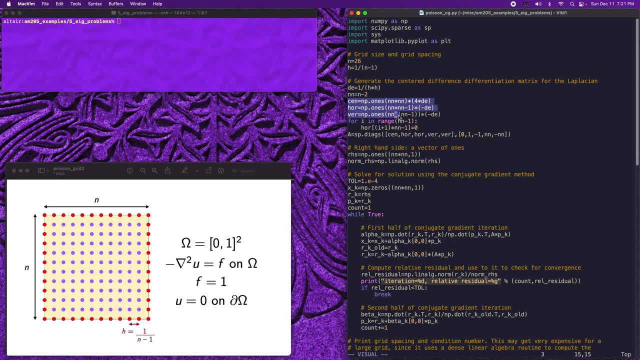 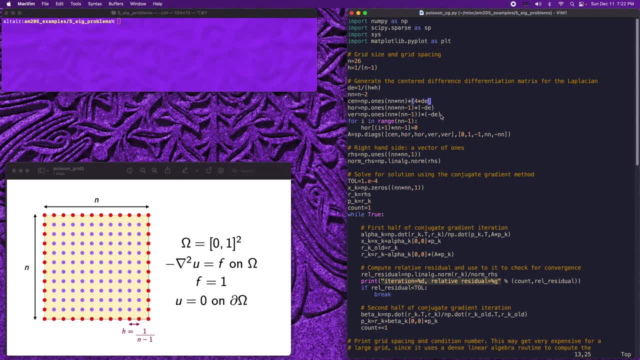 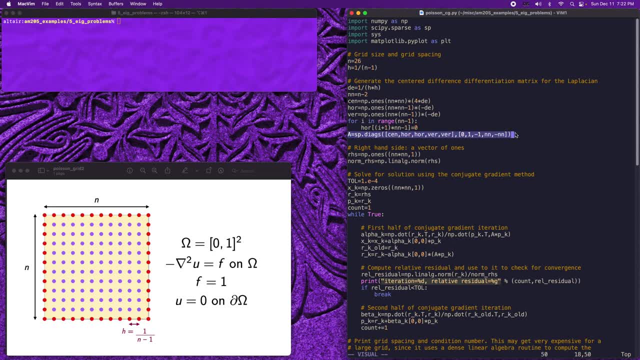 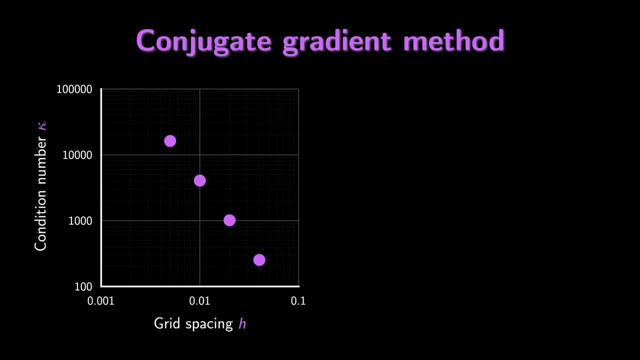 We'll have a central diagonal for our central stencil entries and then four terms corresponding to the diagonal. We'll first look at how the condition number scales as a function of the grid spacing and we'll make use of a log-log pair of axes And we can see that our grid points follow a straight line and if we fit the slope of this straight line then we can indeed verify that the condition number scales like h to the minus 2.. 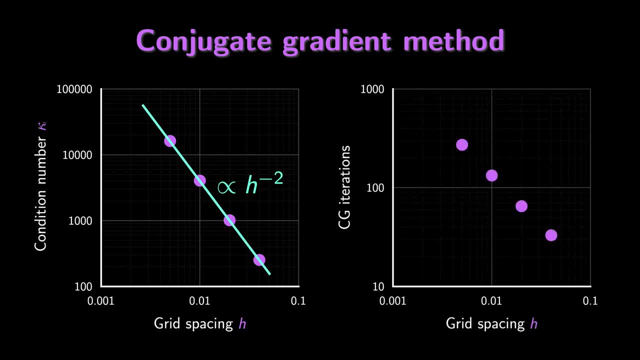 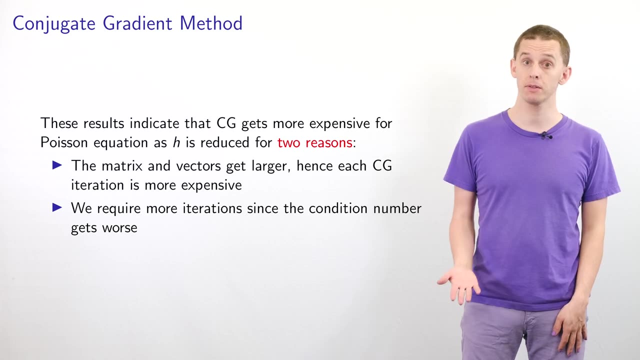 If we look at the number of conjugated iterations required again in log-log space, the points follow a straight line. If we fit these data points, then we indeed see the expected scaling of h to the minus 1.. In the Python example we saw that CG gets more expensive for the Poisson equation as the grid spacing. h is reduced for two reasons. 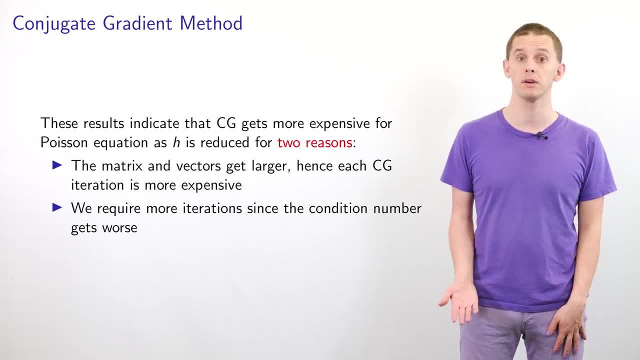 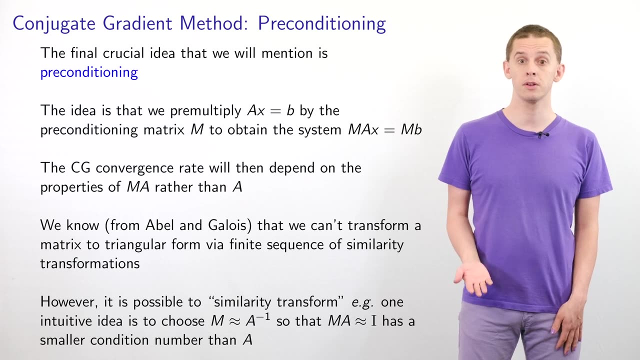 Firstly, the matrix and vectors become larger and therefore each CG iteration is more expensive. In addition, we require more iterations since the condition number gets worse. The final crucial idea that we'll mention is preconditioning, And the idea is that we can premultiply our linear system A is equal B by a preconditioning matrix M to obtain the linear system M A, X equal M B, where the solution X will be the same as for the original system. 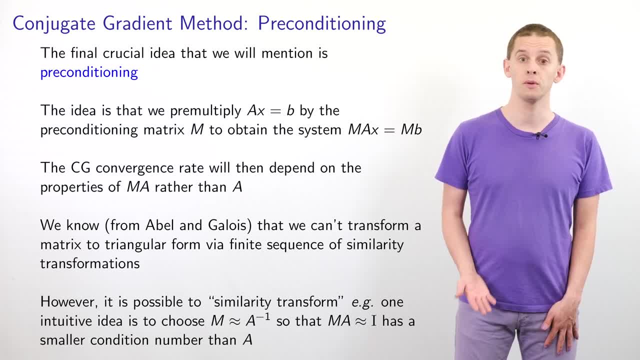 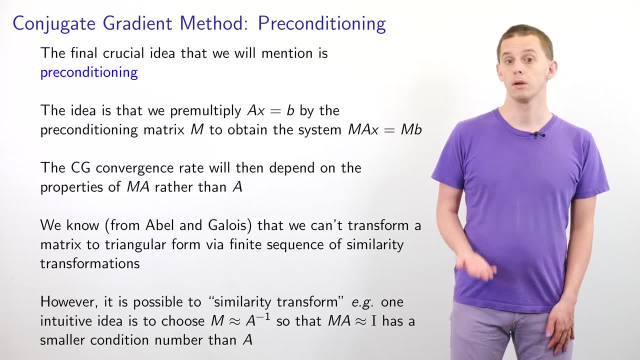 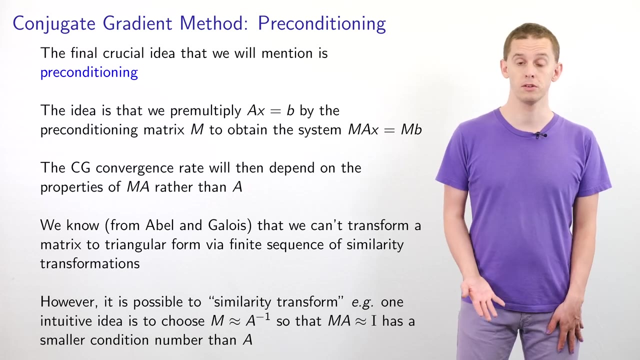 The CG convergence rate will then depend on the properties of M, A rather than A. We know that we need to be able to do this. We know that we can't transform a matrix to triangular form via a finite sequence of similarity transformations. However, it is possible to approximately do this. 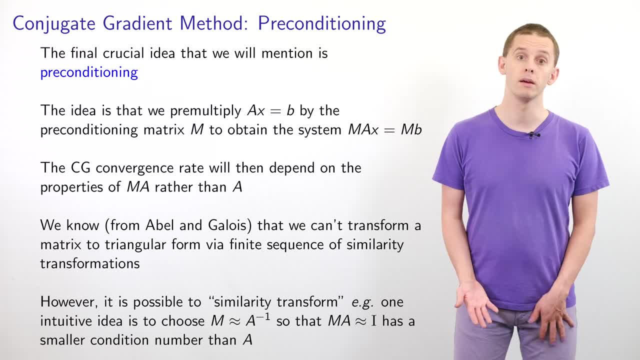 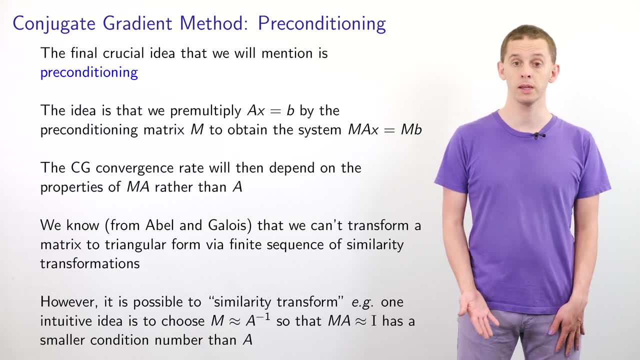 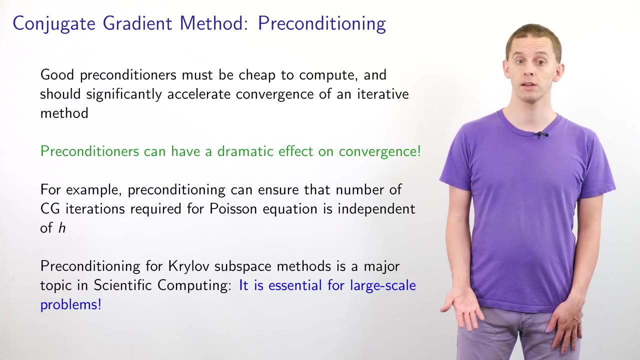 And one idea is to choose M to be the approximate inverse of A And in that case M A will be approximately equal to the identity matrix And that will have a smaller condition number than A. Good preconditioners have to be cheap to compute and they should significantly accelerate the convergence of an iterative method.